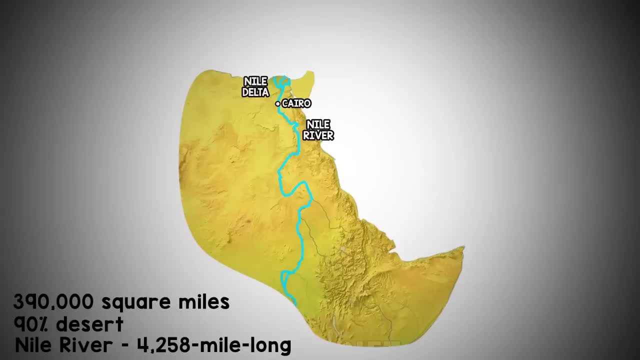 and Who Lived in Ancient Egypt. 3. Geography Shaped the Lives of Ancient Egypt and Who Lived in Ancient Egypt. The Nile Delta has only about 8 inches of rain each year. Due to the fact that it flowed into the Mediterranean Sea, the Nile became a link to an outstanding water trade route. 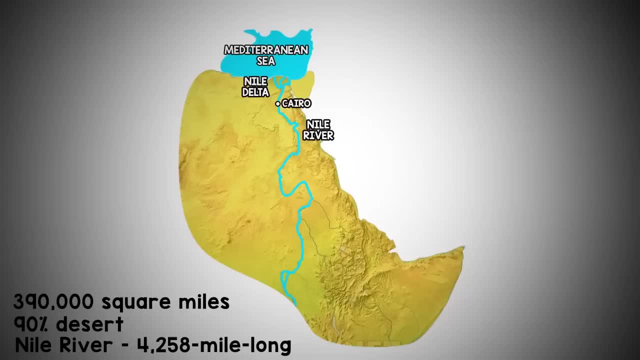 connecting Africa with Europe and Asia. 4. Geography Shaped the Lives of Ancient Egyptians and Who Lived in Ancient Egypt. To the west of the Nile River is the Nubian Desert. The Nile's first natural cataract or shallow area fall within the Nubian region. The Nubian Desert is considered a smaller 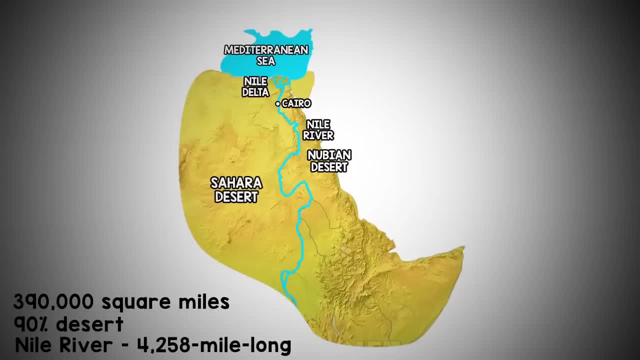 part of the vast Sahara Desert just below Upper Egypt, which is south of Cairo. south of Cairo, The Nile is fed from two rivers in the south of what is now Sudan. The Blue Nile stems from the Ethiopian highlands along the Red Sea, while the White Nile makes the other branch. 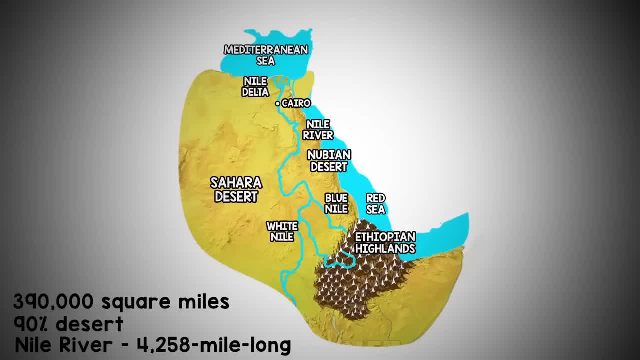 getting its name from the color of the clay it washes. north South of the White Nile River sits Lake Nasser, one of the largest man-made lakes in the world. at 600 feet deep, That's like stacking 60 school buses on top of each other. The Suez Canal drains into a lake in the Nile Delta and 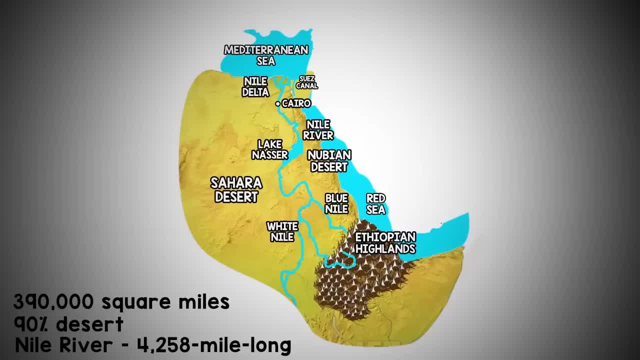 runs southeast all the way to the Red Sea. This allowed watercraft to make their way to the Indian Ocean much faster than circling the African continent. This canal shortens this trip by over 4,300 miles. Egypt and the Red Sea to the east offer a land bridge between Africa and Asia. 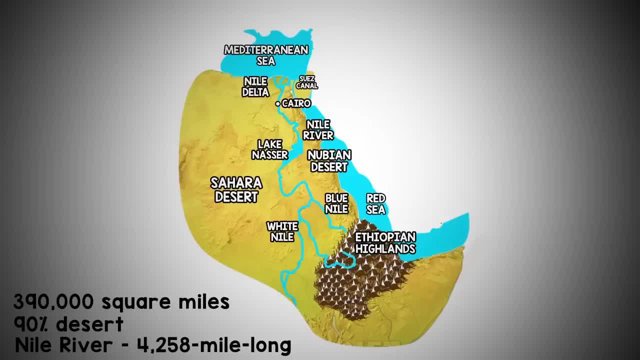 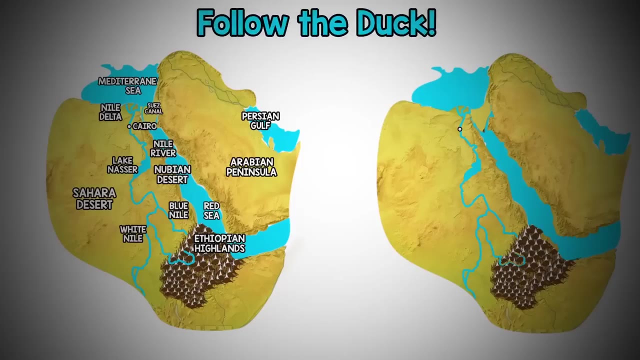 Ancient merchants and pilgrims traveled from the Nile River Valley north, past the Red Sea, crossed the Arabian Peninsula and then rounded the Persian Gulf. Test your knowledge, Let's play Where's the Duck? In this game, you will track the duck. 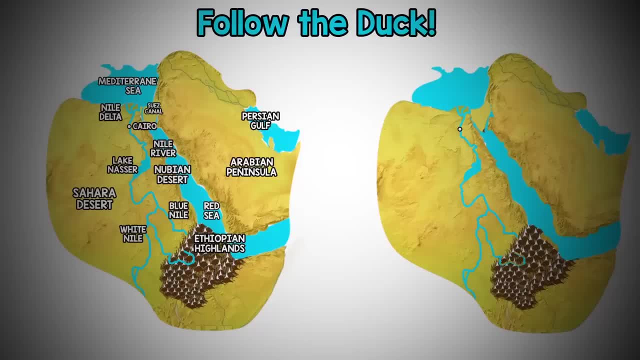 as it appears on a blank map of Egypt. Once the music stops, you will use an Egypt map labeled with physical features to determine where the duck ended up. Other animals may appear On the map, so don't forget to keep your eyes on the duck. 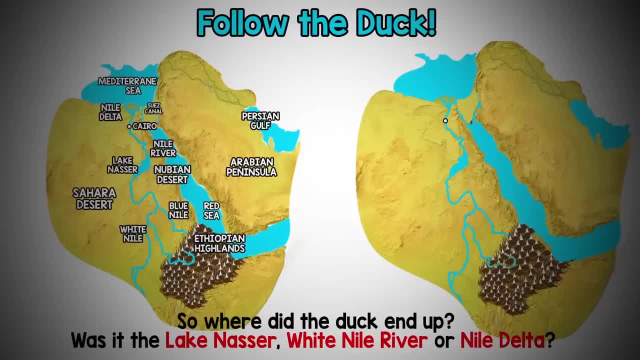 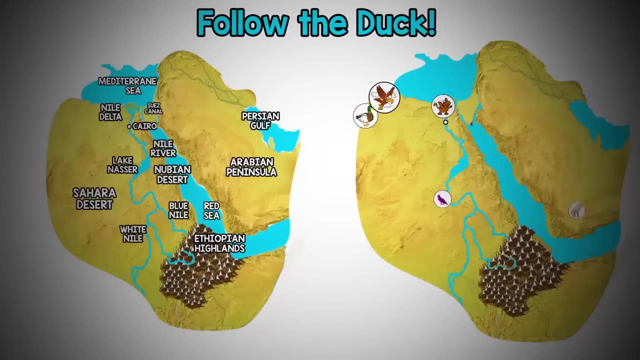 So where did the duck end up? Was it Lake Nasser, the White Nile River or the Nile Delta? That's right, it was Lake Nasser. Let's try it again. Remember to keep your eyes on the duck. So where did the duck end up? Was it the Nile River, the Red Sea or the Nubian Desert? 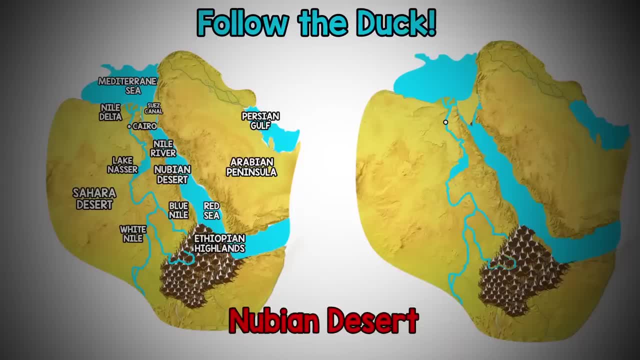 That's right, it was the Nubian Desert. So where did the duck end up? Was it the Nile River, the Red Sea or the Nubian Desert? Let's try one last time. You got this. So where did the duck end up? Was it the Ethiopian Highlands, the Sahara Desert or Lower Egypt? 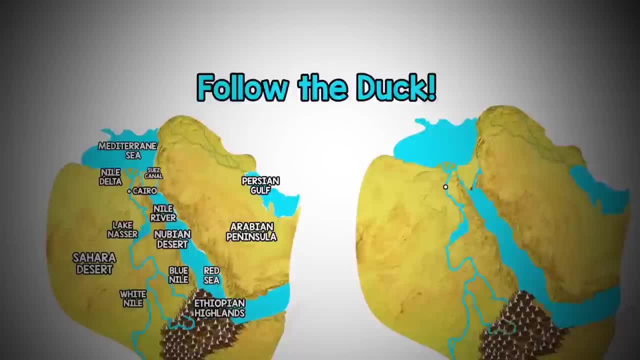 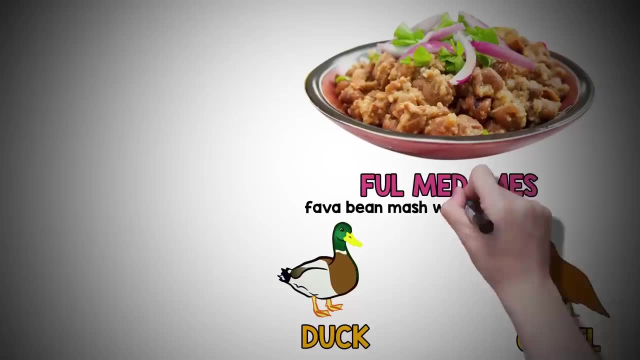 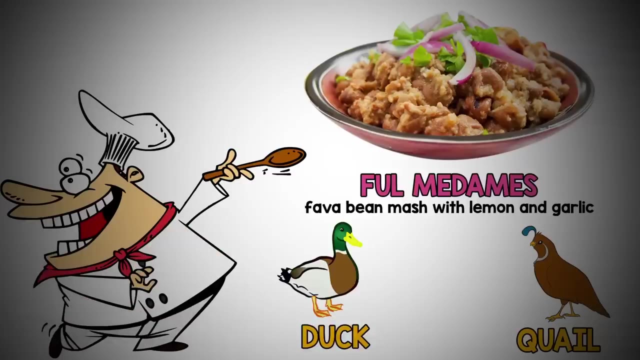 Nice job, It was the Sahara Desert. Here's the dish. In addition to duck and quail, a popular Egyptian meal is called ful mudamas, which was a fava bean mash with lemon and garlic. Originally, the Egyptians prepared this meal in a pot that they buried in desert sand. 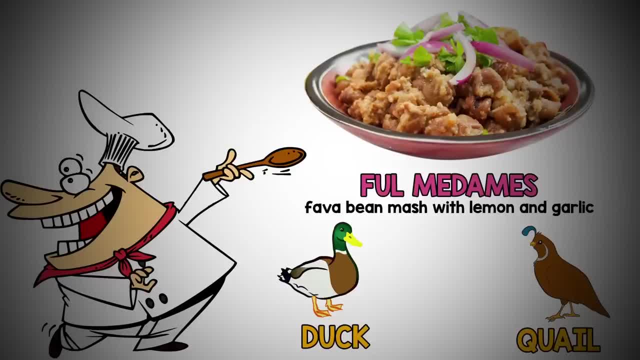 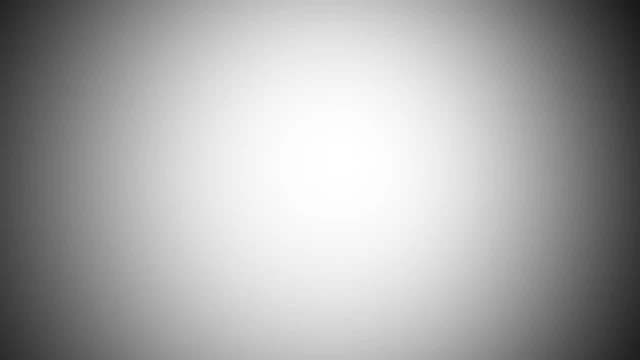 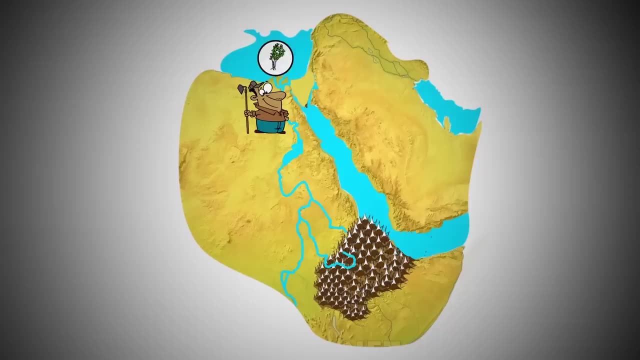 The heat of the sand covering it cooked the mash like an ancient crockpot. How does geography shape lives? The Nile River equaled life for the Egyptians. They farmed on the Nile's banks. Healthy crops of barley and other grains thrived in its rich soil. 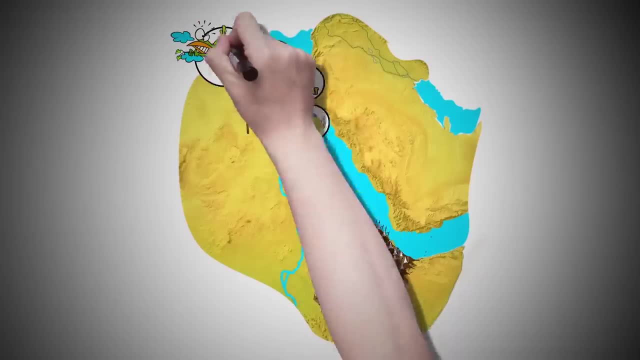 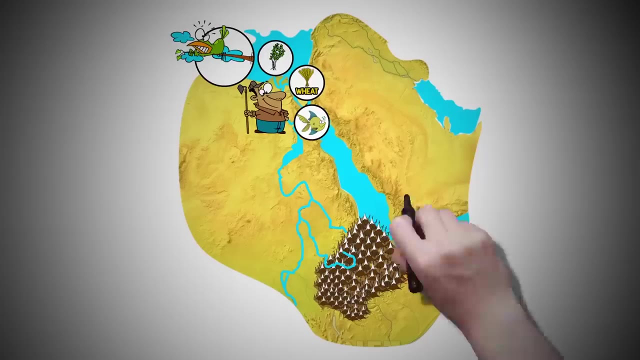 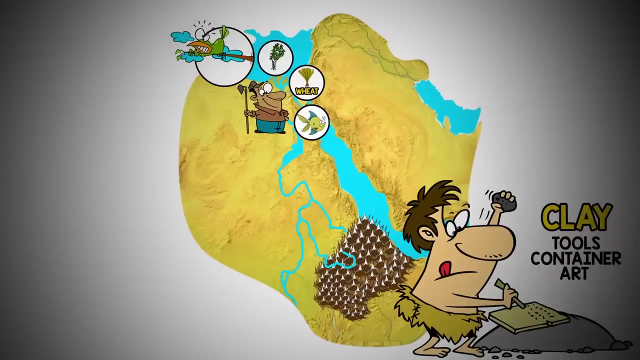 The fish and small birds that lived in and around the Nile also offered food for the Egyptians. Legends and religion stemmed from the Nile and its surrounding landscape. Clay from various stretches of the Nile River became useful tools and containers, as well as art. Flax was also grown in Egypt and, when dried and spun, became linen cloth. 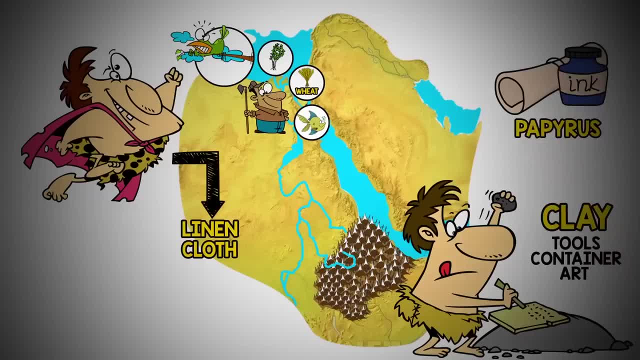 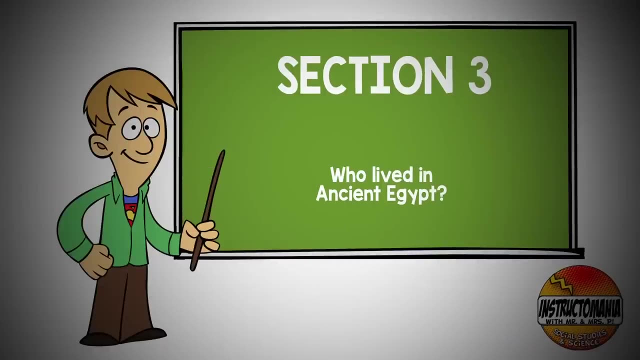 Papyrus was treated the same way as flax and dried into paper. The Nile River Valley also provided mines of copper, which they made into tools and traded for other needed resources from Egypt's neighbors Who lived in ancient Egypt- Hunter-gatherer nomads settled along the Nile River. 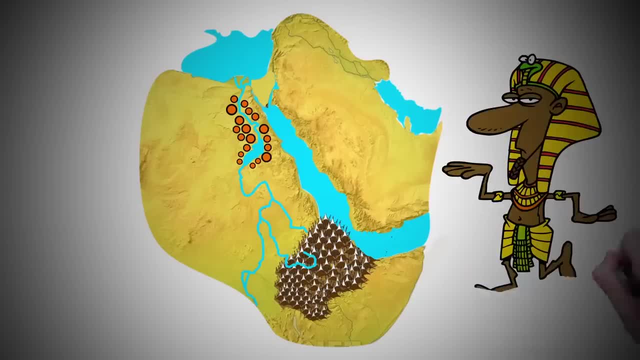 starting around 6,000 BCE, and the written history of Egypt started when it was unified by Menes, around 3,150 BCE. The Intermediary Period marked a split in Egyptian government when two major capitals arose: Thebes in Upper Egypt and Hierakonpolis in Lower Egypt. 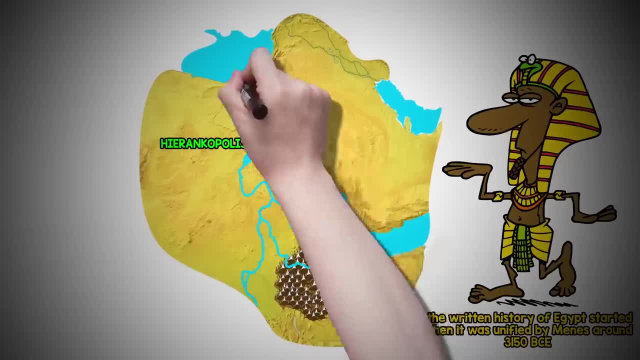 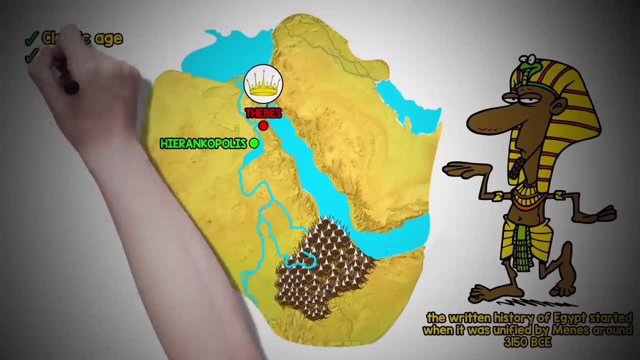 Thebes eventually overtook Hierakonpolis and started a dynastic rule, moving Egypt into the Classic Age. Art, culture, science and farming techniques greatly expanded during this time. Then Thebes weakened enough for invaders to take over. 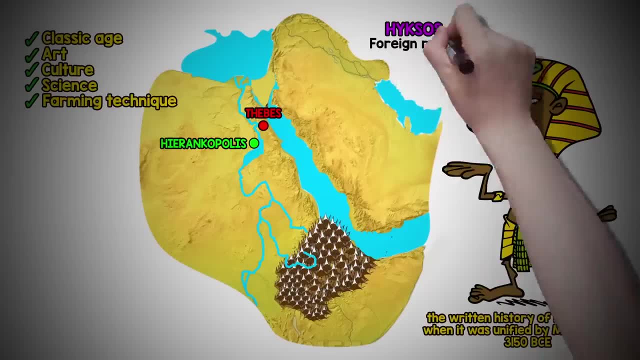 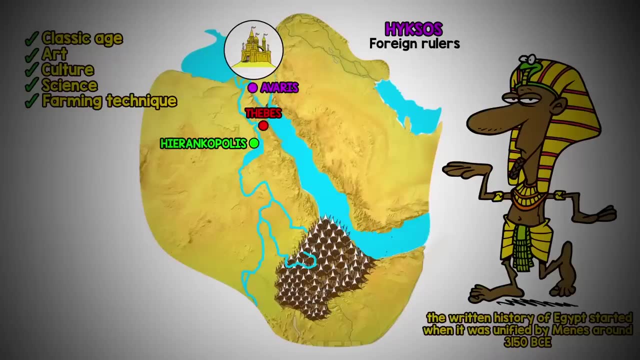 Little is known about Hyksos, meaning foreign rulers, except that they gained a stronghold in the city of Avaris and spoke a Semitic language similar to that in Middle Eastern countries. At the same time, the Nubians also took over southern Egypt. 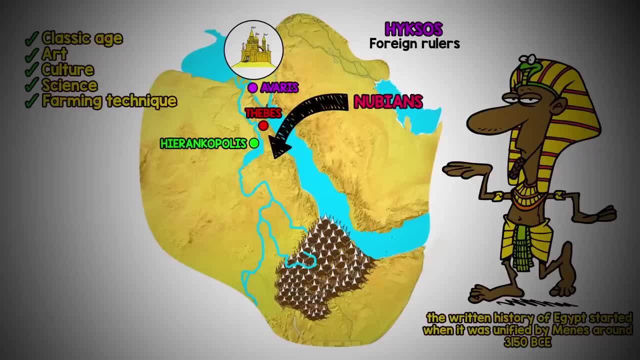 Both cultures melded with Egyptian culture, causing a rich and diverse country. Eventually, Egyptians regained their lands and continued dynasty-based rule until Egypt was conquered by the Greeks. Later, Islam would greatly affect the people of Egypt as Muslims spread over and settled in Northern Africa. 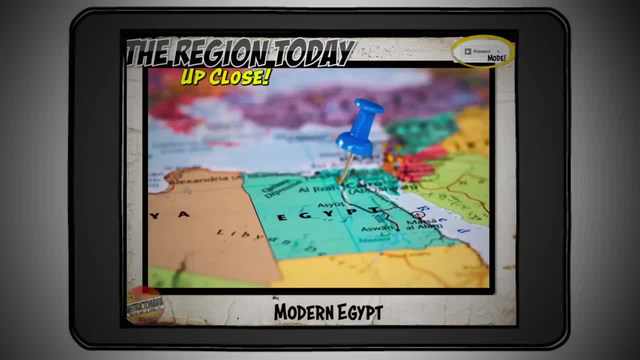 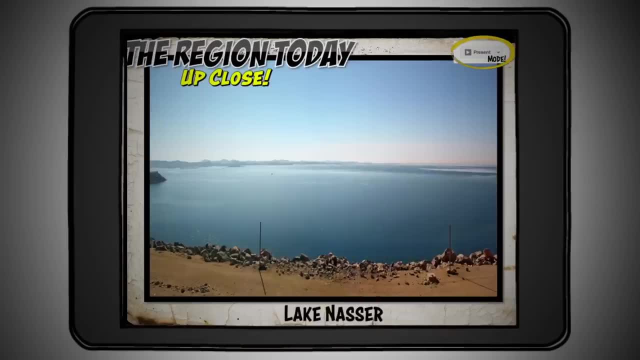 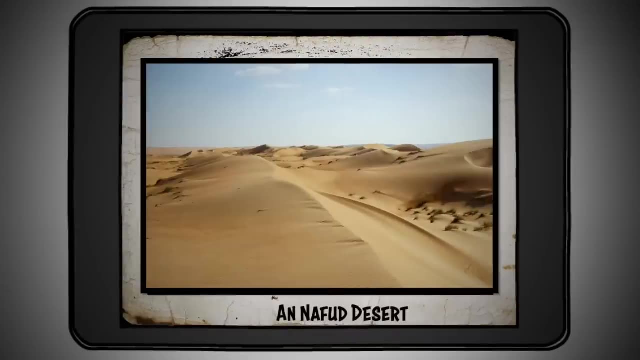 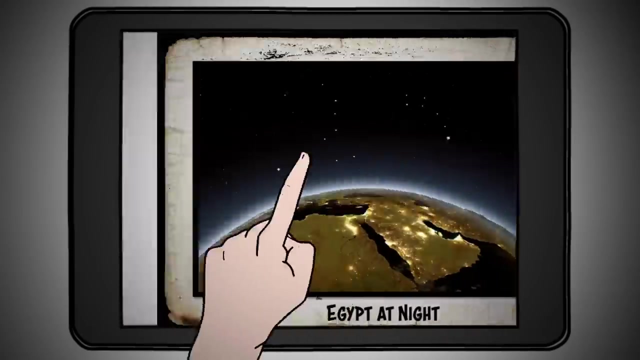 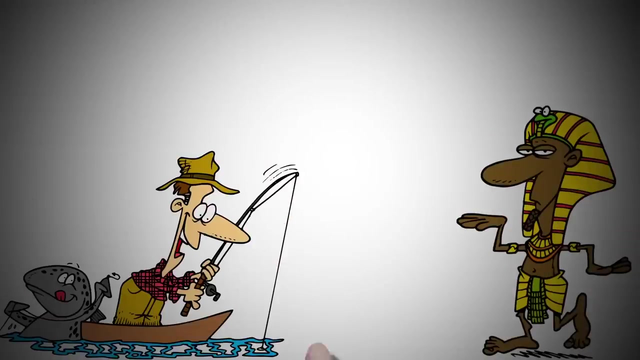 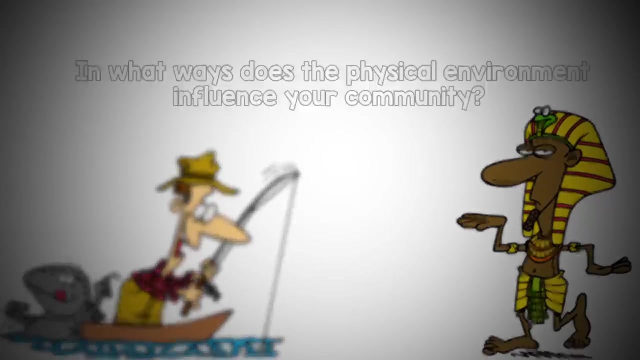